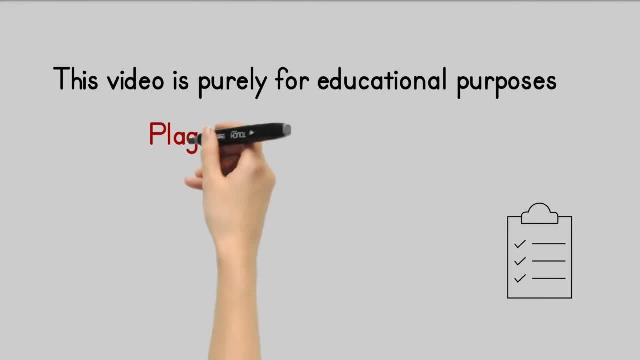 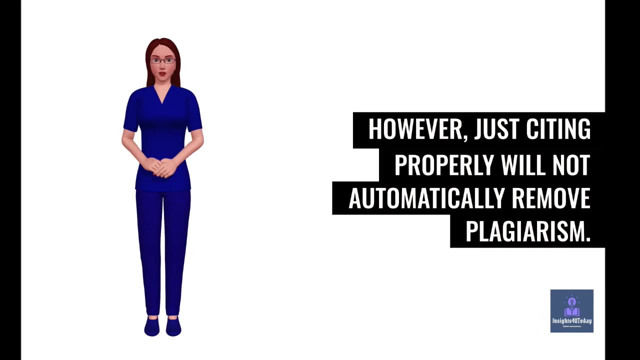 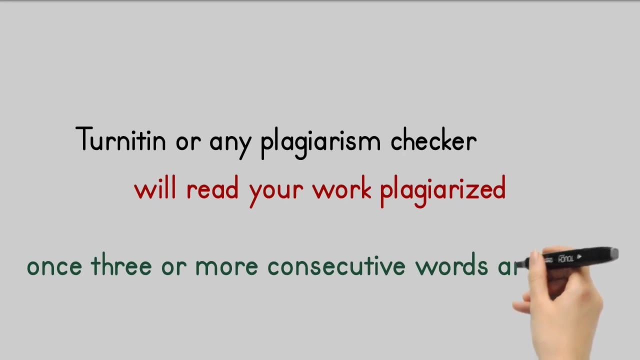 Remember this video is purely for educational purposes. Plagiarism is very unethical. You must cite all sources used. However, just citing properly will not automatically remove plagiarism. Turnitin or any plagiarism checker will read your work plagiarized once three or more consecutive words are seen in your documents. 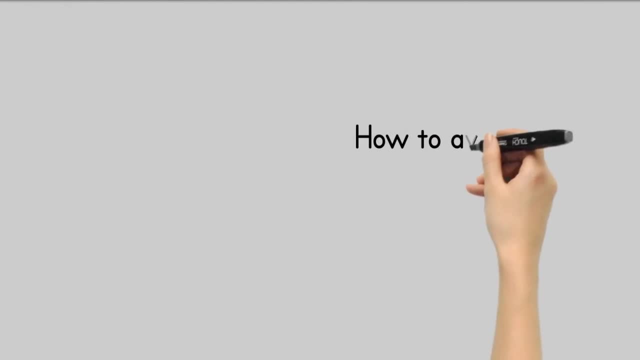 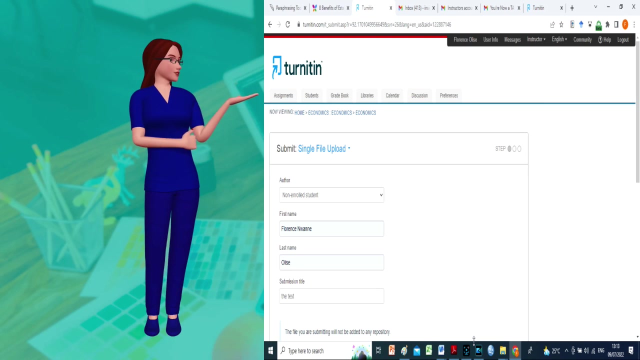 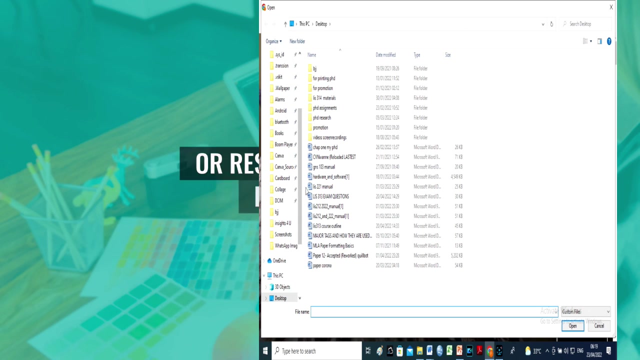 Yet it would be best if you referred to the existing literature in any academic writing or research. How, then, can we avoid plagiarism, even while citing? I will show you how to avoid or remove plagiarism using four simple steps. If you follow these steps carefully, no plagiarism checker, not even Turnitin Plagiarism Checker X or Inago Plagiarism Checker- will read your reports, essays or research papers as plagiarized. 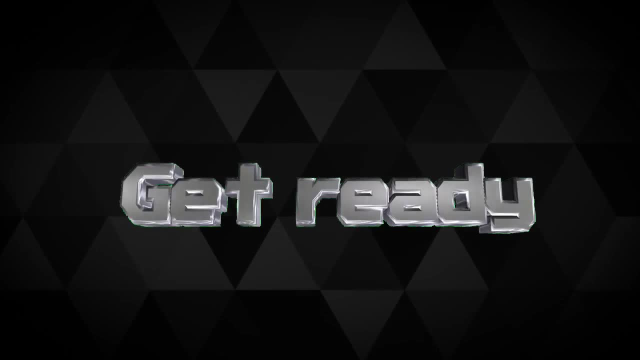 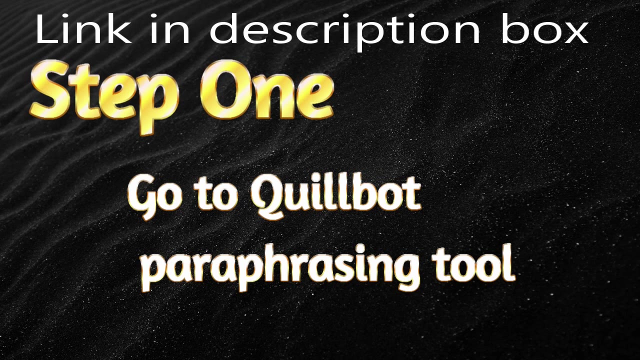 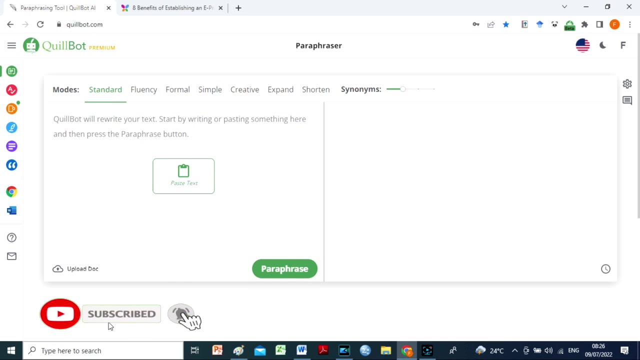 Are you ready? Let us get to it now. Step 1. Go to the Quillbot paraphrasing tool. The link is in the description box below. You cannot pass any plagiarism test without paraphrasing. If you paraphrase using Quillbot the usual way, you usually get a similarity index of about 25-30%. 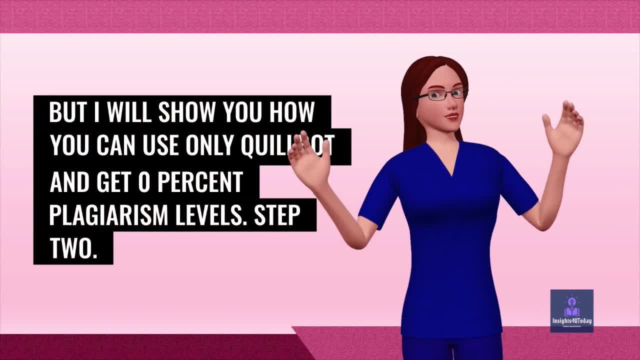 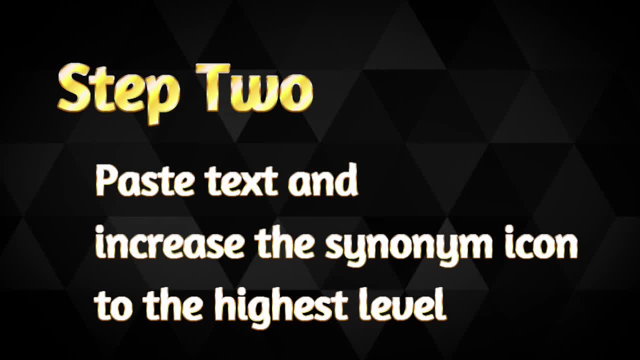 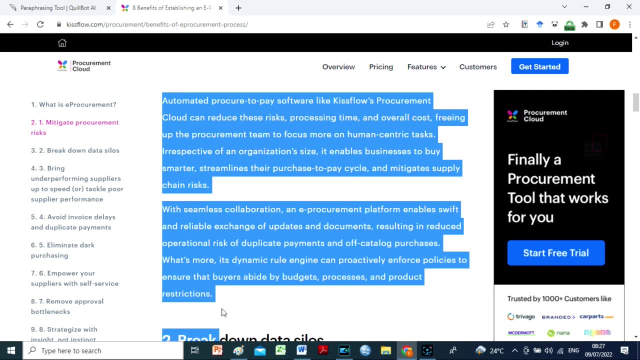 But I will show you how you can use only Quillbot and get 0% plagiarism levels. Step 2. Paste text here. I will copy some text online which will have 100% plagiarism levels. Then increase the synonym icon to the highest level. 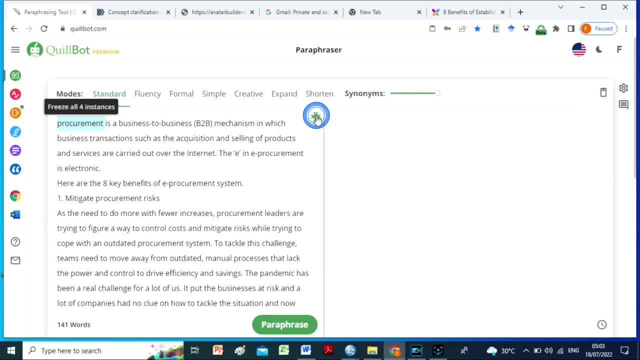 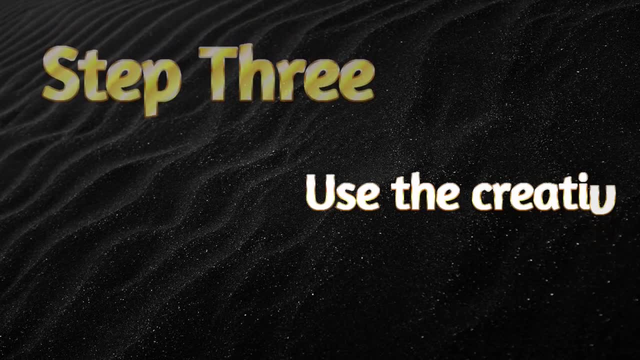 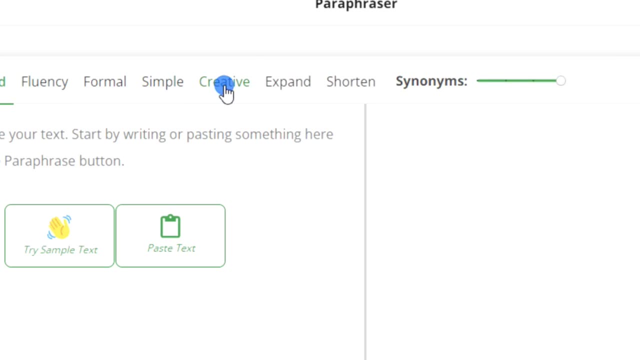 Increasing the synonyms will make your sentence change significantly. However, try to freeze your keywords first over here. I will explain more in a short while. Step 3. Use the Creative Mode. The Creative Mode usually changes the sentence structure while paraphrasing, but does not change the meaning. 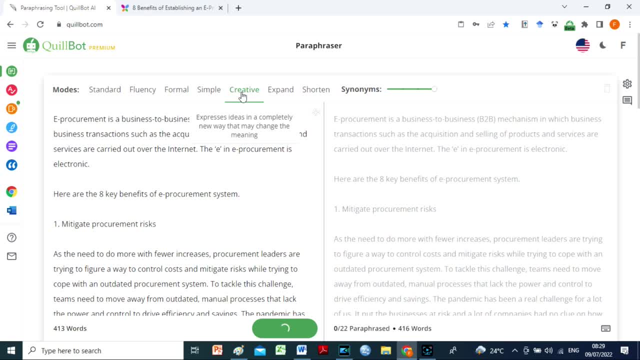 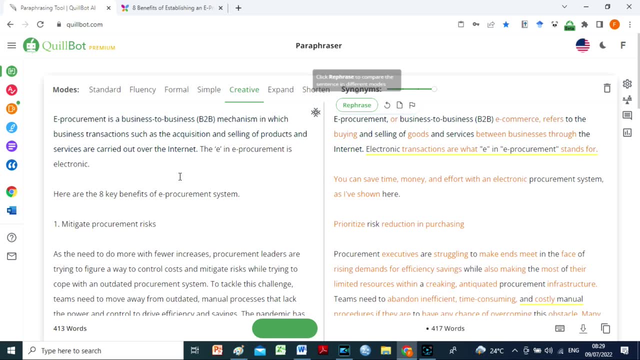 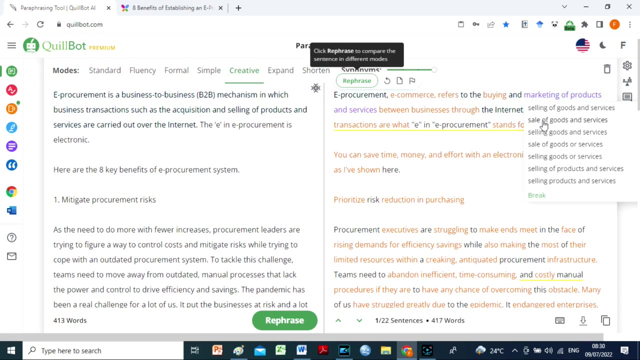 You need to understand that any good plagiarism checker will read any three or more consecutive words not changed as plagiarized. Therefore, look at the result, the paraphrased text, and try to replace synonyms of words in black and blue colors too. Words in blue show the longest unchanged words. 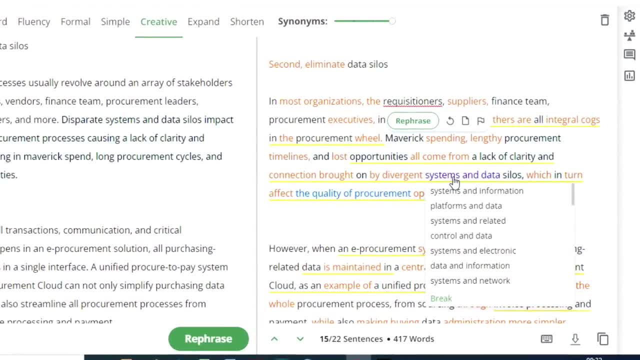 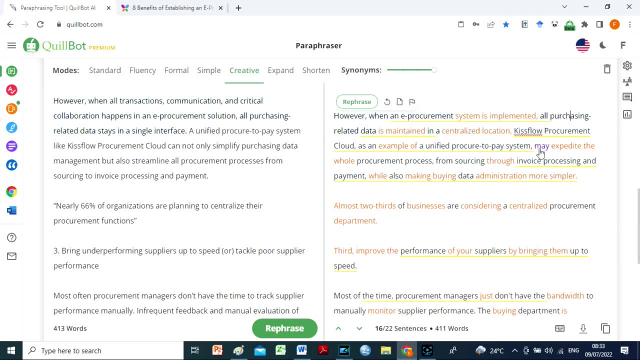 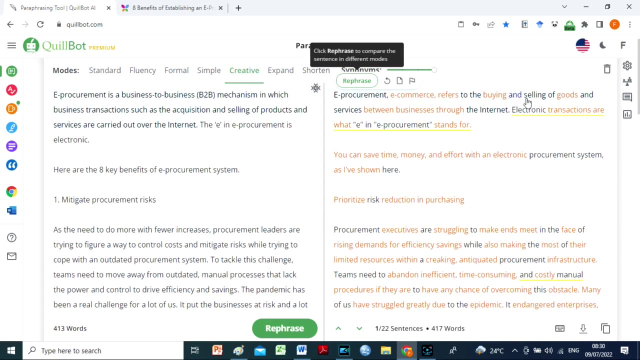 Turnipin is going to read them as plagiarized. You can rephrase any sentence you don't like. like this using any mode of your choice. The black texts have not to be changed. It would help if you work towards getting more red words. 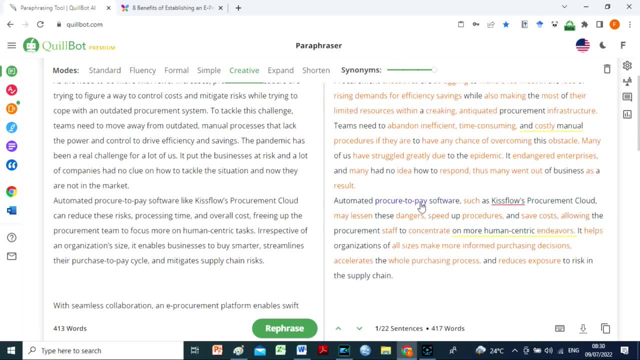 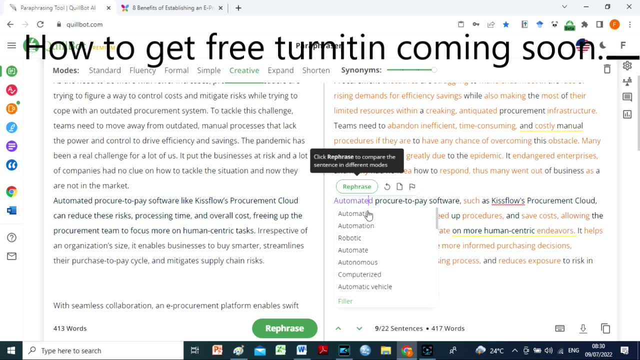 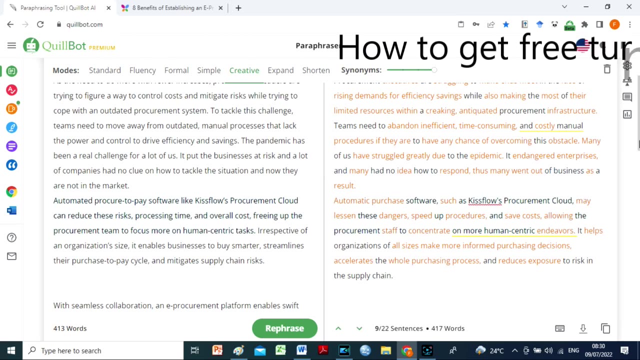 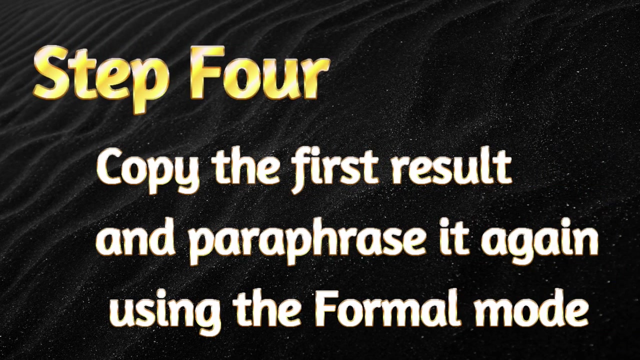 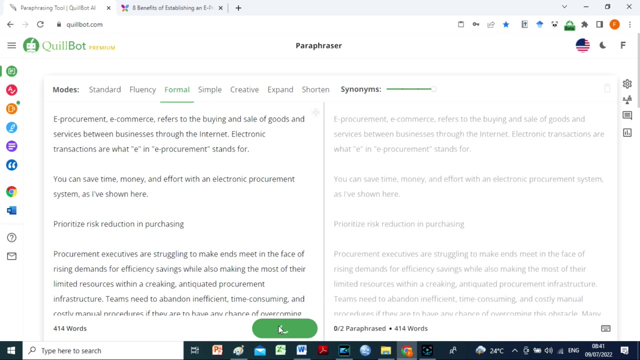 So choose the best synonyms that suit your objective. Step 4. Copy the first result and paraphrase it using the Formal Mode. This will make your writing sound very formal and professional. However, if you want to sound creative, you can paraphrase again using the Creative Mode. 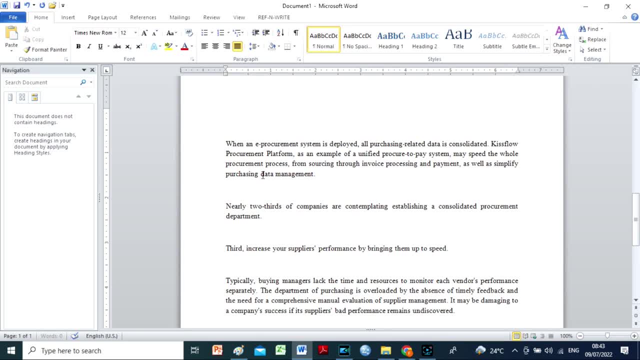 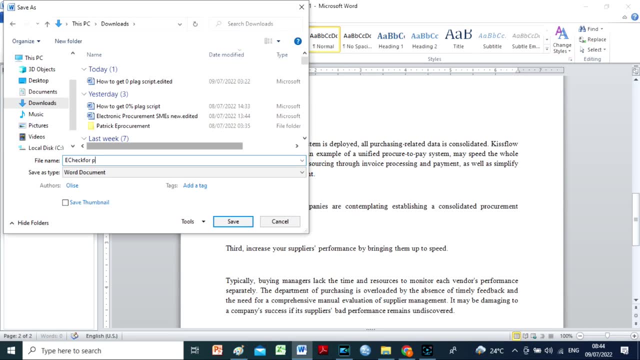 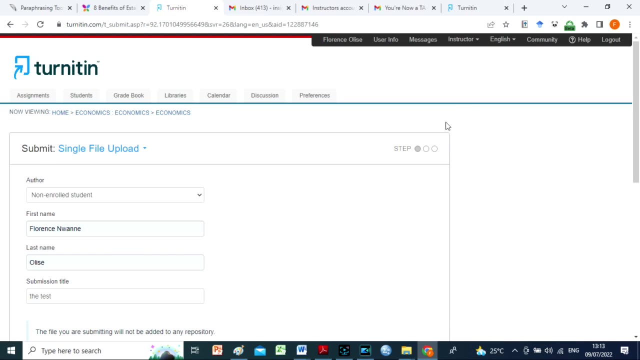 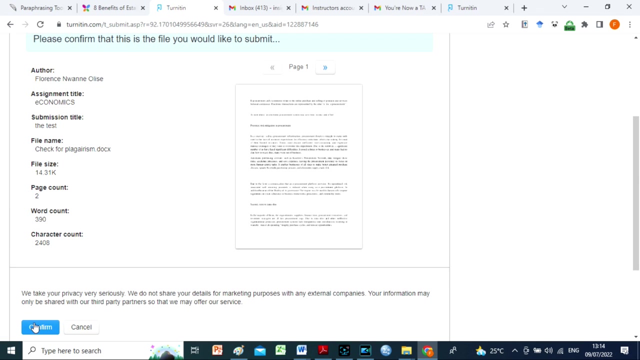 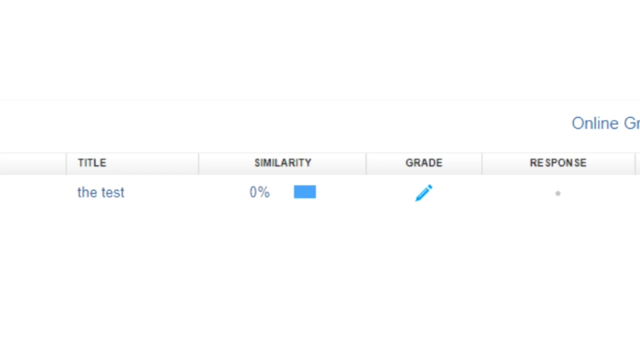 Then we will check for plagiarism. Always check your writings for plagiarism Before final submission or publishing. it is time to conduct a plagiarism test for our paraphrased text. using Turnipin. Here we are: 0% similarity index- Awesome. 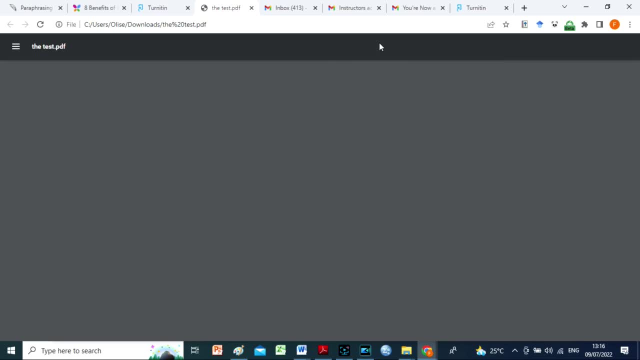 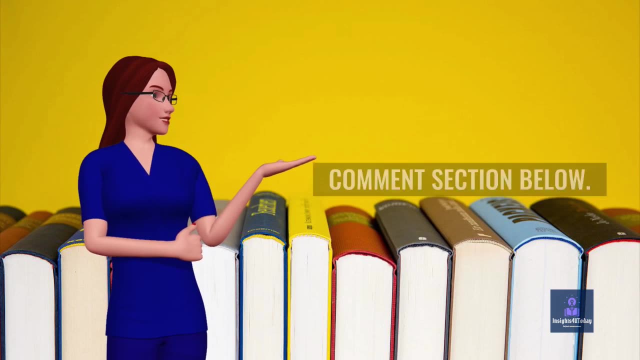 Right. If this plagiarism removing trick is helpful to you, please share this video, hit the like button and write no more plagiarism in the comment section below. If you want to continuously get a free Turnipin class ID and enrollment key for your plagiarism test, check the link in the description box. 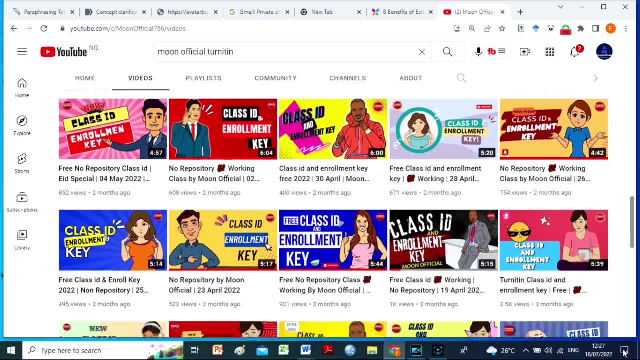 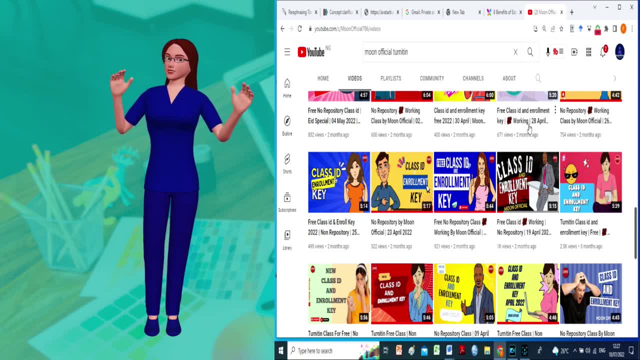 It is from a YouTuber called Moon Official. He posts videos on working class IDs and enrollment keys without a repository on YouTube every two or three days. Trust me, He is the best you can find on YouTube. This is not a sponsored message. 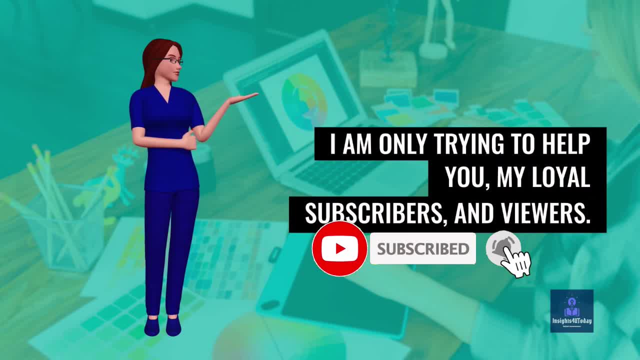 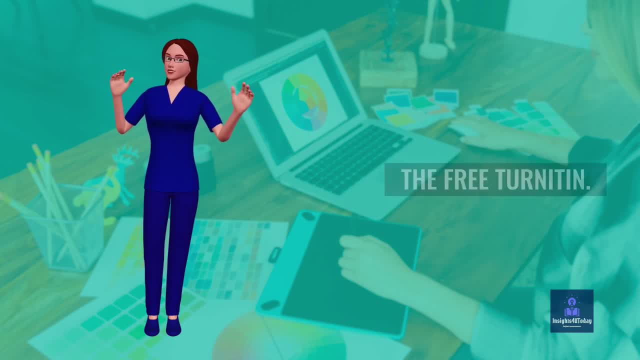 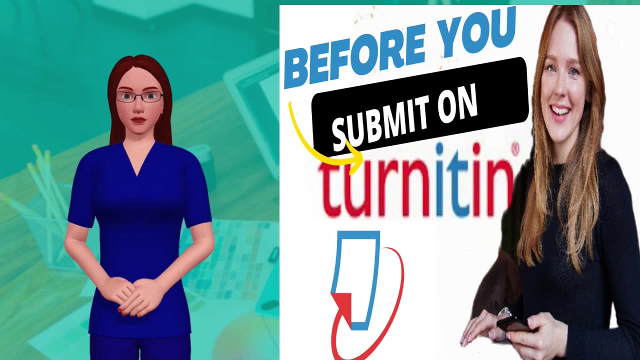 I am only trying to help you, my loyal subscribers and viewers. I recommend you subscribe to his channel and hit the notification bell so that you can be among the first to get the free Turnipin. If you don't know how to use the free class ID and enrollment key Moon Official provides, see my video on 5 things you must do before submitting to Turnipin, suggested in the description box.